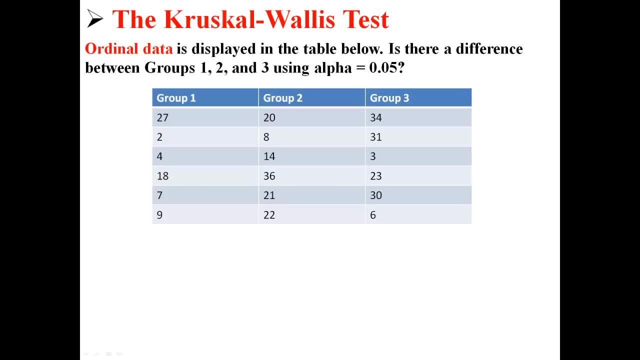 scores for each group. Is there a difference between groups 1,, 2, and 3 using an alpha level of 0.05?? We're going to perform a Kruskal-Wallis test on this data set to see if there's a 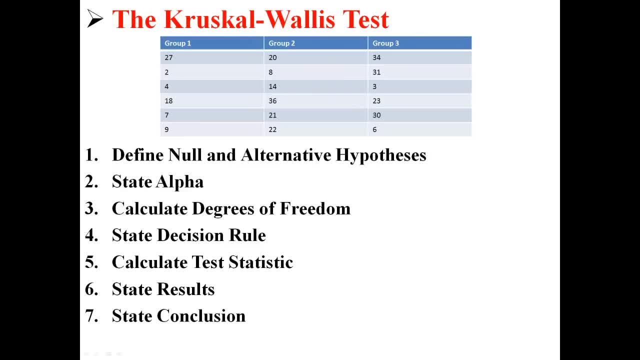 difference between the three groups. Our Kruskal-Wallis test has seven steps. First we're going to define what our null and alternative hypotheses are. next we're going to state our alpha. then we're going to calculate our degrees of freedom. then we state our decision rule. then we 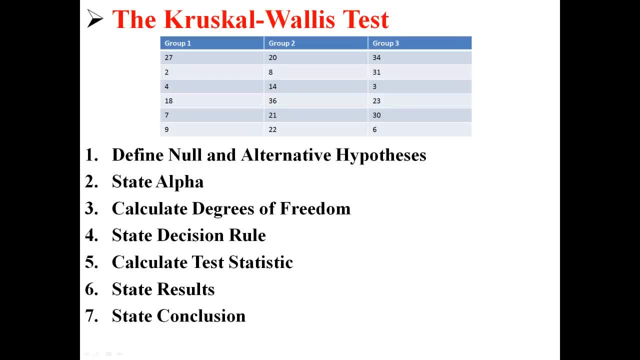 actually calculate the test statistic and then, finally, we state our results and our conclusion. So let's start with step one, defining the null and alternative hypotheses For a Kruskal-Wallis test. our null hypothesis- H0, is that there is no difference between the treatments that we're 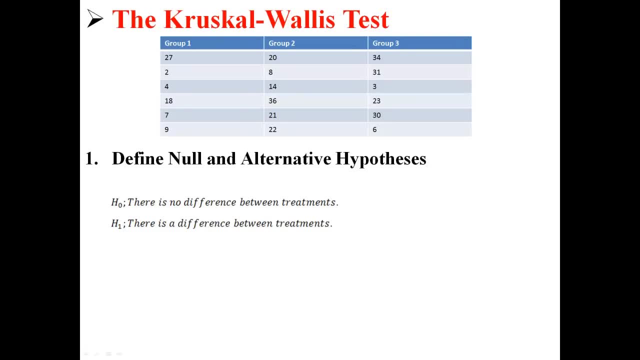 comparing Our alternative hypothesis H1, is that there is a difference between the treatments that we are comparing. Step two is to state the alpha level. That's easy because, I already said, use an alpha level of 0.05.. Next we're going to calculate our degrees of freedom. 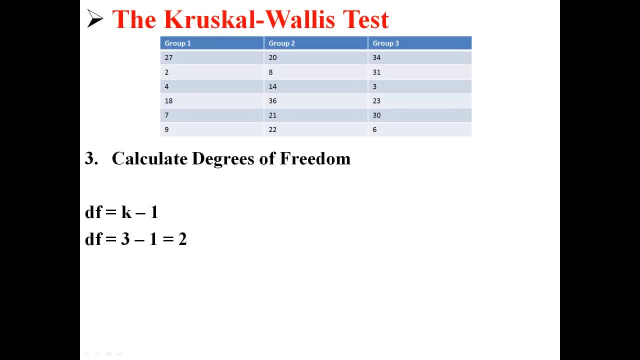 Degrees of freedom are equal to k-1,, where k is the number of groups you have. So in this case, our degrees of freedom is equal to 3-1, or 2.. Next, based on that information, we state our decision. 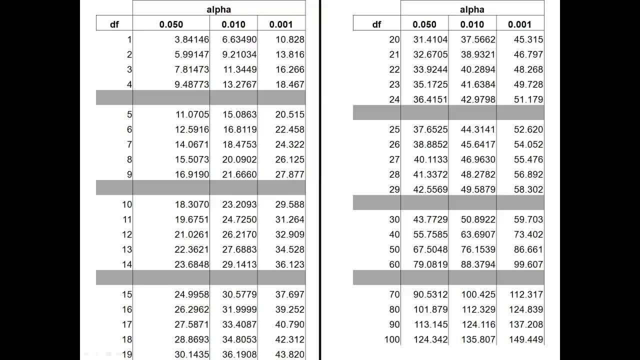 rule. Here we go to our chi-square table, which is what we use for a Kruskal-Wallis test. We have an alpha level of 0.05 and two degrees of freedom. Using that information, we can find our critical value Here. our critical value is 5.99147.. 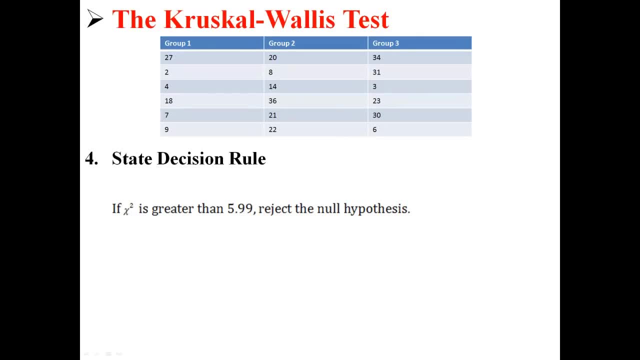 So if the chi-square value that we calculate is greater than 5.99, we can reject the null hypothesis and say that there is a difference somewhere between the three groups. If chi-square is not greater than 5.99,, then we will not reject the null hypothesis. Now let's actually calculate. 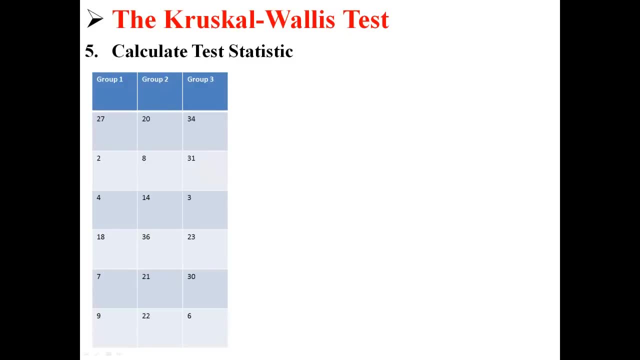 our test statistic. Here we have our information- I just moved it over to the left so we can work with it- And what we want to do for a Kruskal-Wallis test is organize our scores by rank. So basically we want to organize them from smallest to largest. Here we have three groups with six. 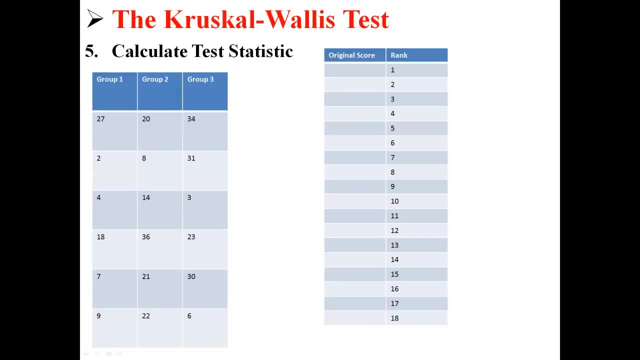 scores in each group, so we have 18 scores. We're going to rank those 18 scores so we can calculate the chi-square statistic for our Kruskal-Wallis test Here we've just taken the original scores and ranked them. For example, our smallest score is 2, so that's rank 1,. 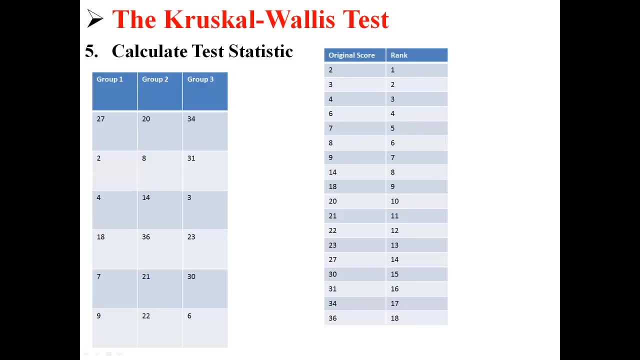 while our largest score is 36,, so that's rank 18.. So now I've changed the table to reflect that We're no longer working with the original data, we're working with our ranks because, remember, our original data is ordinal. 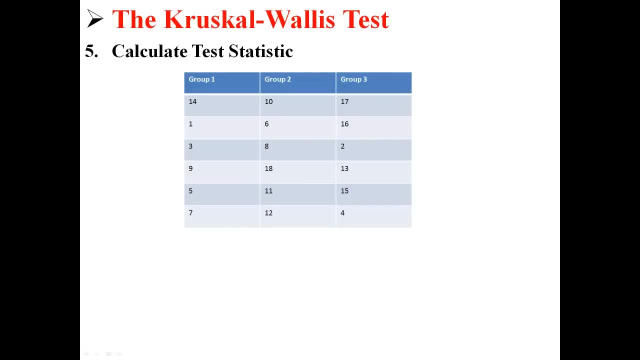 So now we have our table with our ranks. So now we can calculate our test statistic, Our test在. we're going to call it h, but just basically think of it as a chi-square value. And here we have our equation for calculating that. 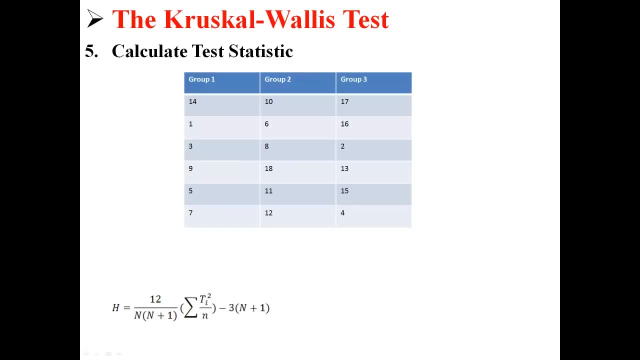 It's this kind of complicated: 12 divided by n times n plus 1 times all of the sum squared, divided by n minus 3 times n plus 1.. That sounds kind of confusing, but I'll show you right now how we actually get those numbers. 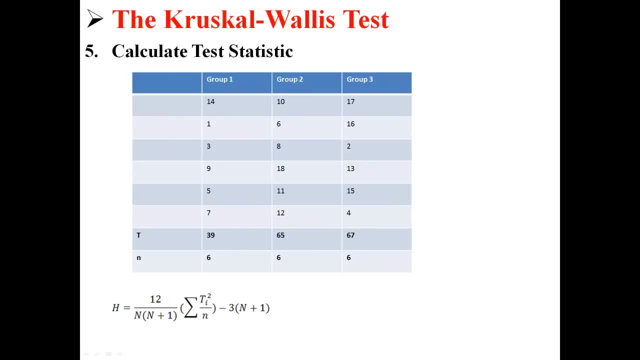 So first our t is our sums. So for example, the sum of group 1 is 39,, the sum of group 2 is 65,, the sum of group 3 is 67. And our n is just our sample sizes. 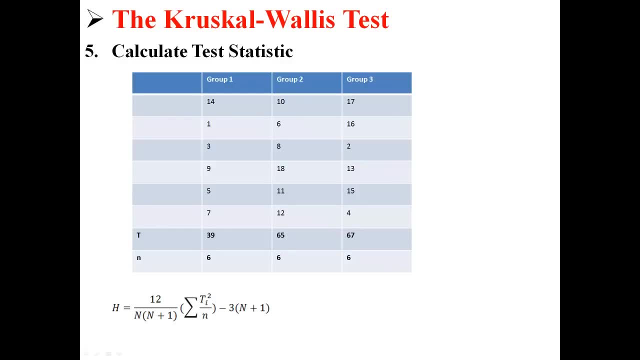 We have 6 scores in each of our groups, in each of our samples, so all of our n's are 6.. So now that we have that, we can just plug those into the equation to solve for h For each t-square. you know t1,, 39,, t2,, 65,, t2, sorry, t3 is 67.. 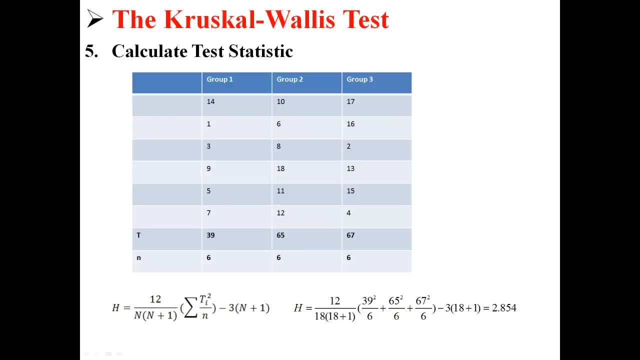 Our big N reflects our total sum, So we have our total sample size. So while each small n is 6, our total sample is 18.. It's just 6 plus 6 plus 6.. And we just plug all of those values into the equation to find our h value of 2.854. 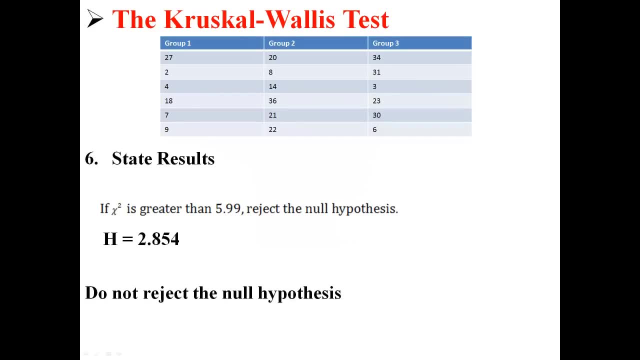 So now we can move on to our results. Remember: our decision rule was: if our chi-square value was greater than 5.99, we were going to reject the null hypothesis. In this case, our value is 2.854.. Because it's not greater than 5.99, we do not reject the null hypothesis.